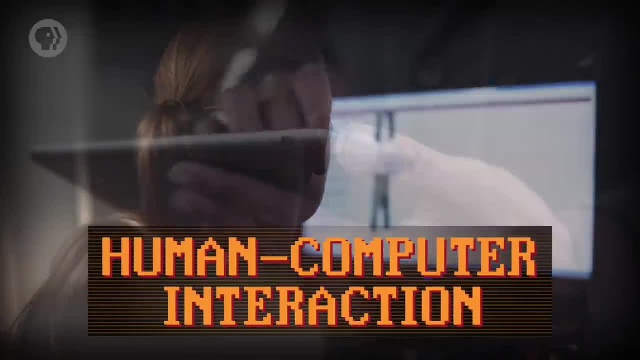 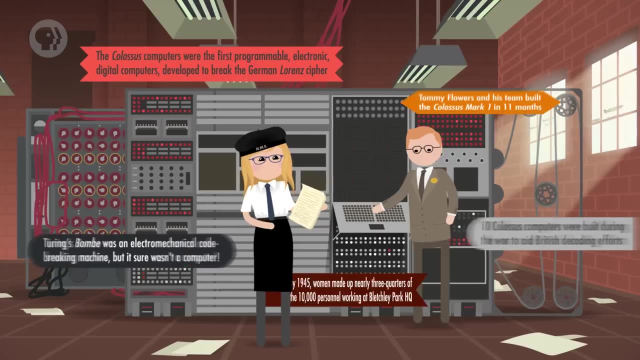 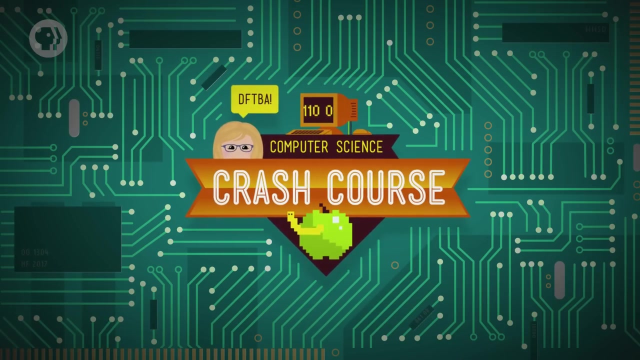 today there's a whole field of study called human-computer interaction. These interfaces are so fundamental to the user experience that they're the focus of the next few episodes. As we discussed at the very beginning of the series, the earliest mechanical and electromechanical. 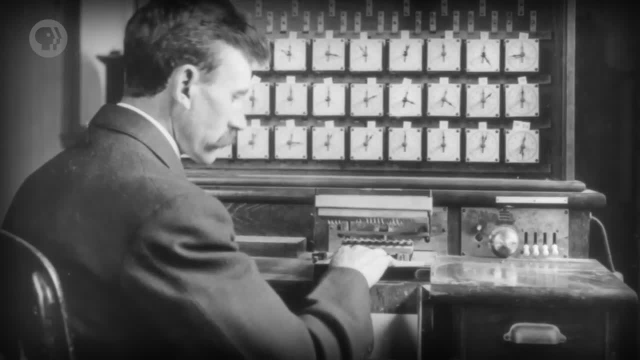 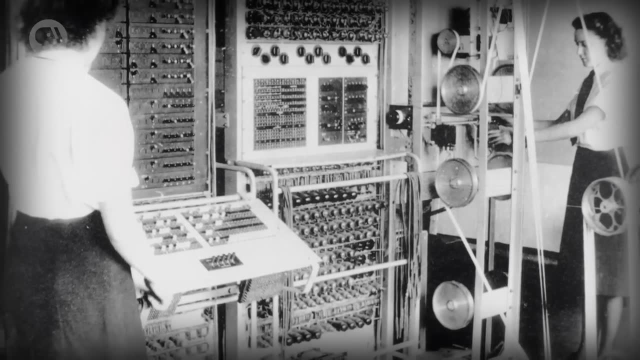 computing devices used physical controls for inputs and outputs, Like gears, knobs and switches, And this was pretty much the extent of the human interface. Even the first electronic computers, like Colossus and ENIAC, were configured using huge panels of mechanical controls and patch wires. It could take weeks to enter in a single. 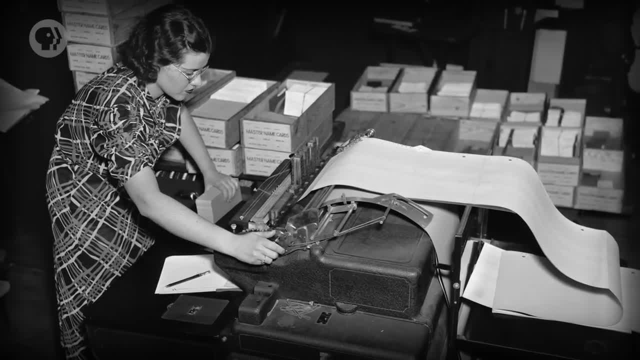 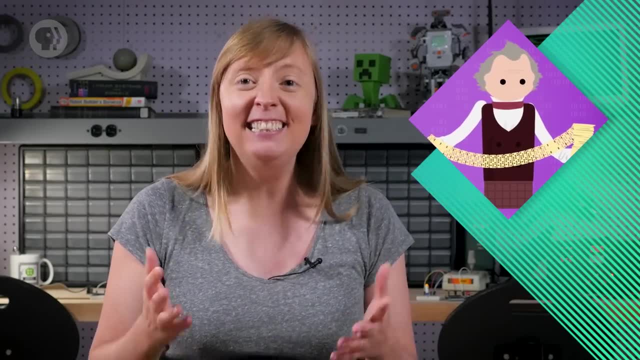 program, let alone run it, And to get data out. after running a program, results were most often printed to paper. Paper printers were so useful that even Babbage designed one for his difference engine, and that was in the 1820s. 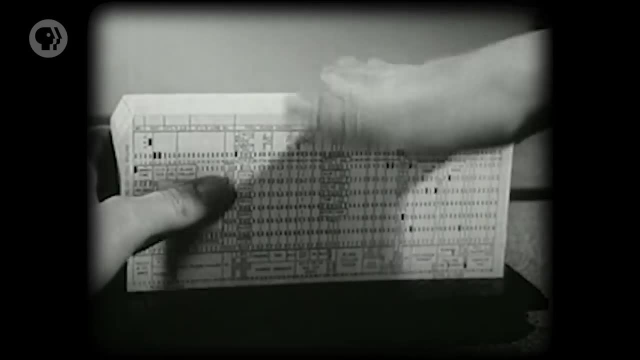 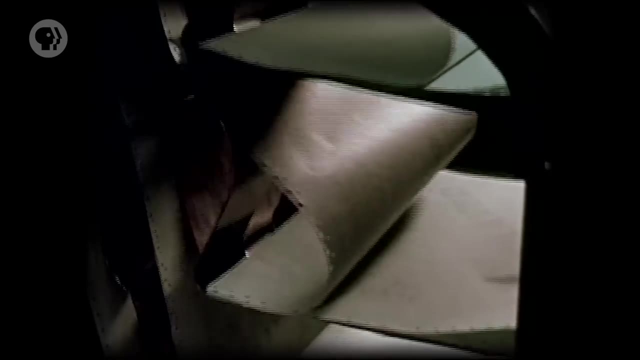 However, by the 1950s, mechanical inputs were rendered obsolete by programs and data stored entirely on mediums like punch cards and magnetic tape. Paper printouts were still used for the final output and huge banks of indicator lights were developed to provide real-time feedback while the program was in progress. 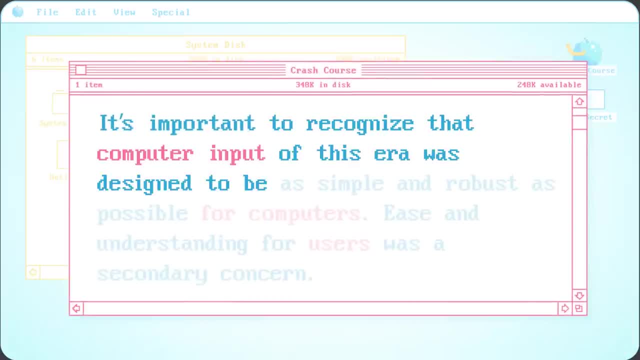 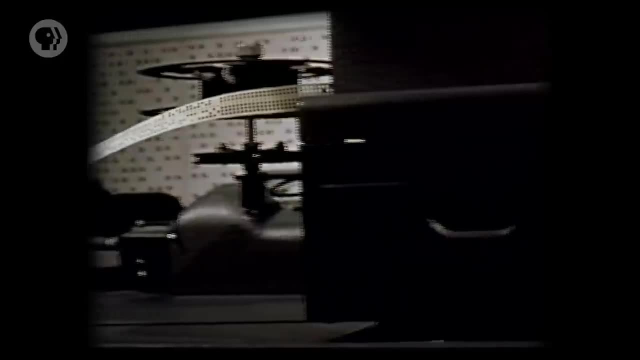 It's important to recognize that computer input of this era was designed to be as simple and robust as possible for computers. Ease and understanding for users was a secondary concern. Punch tape is a great example. This was explicitly designed to be easy for computers to read. 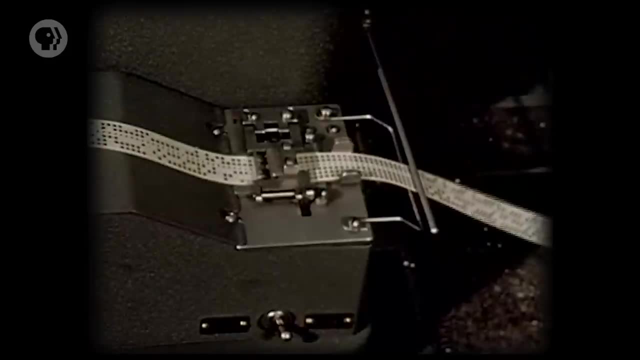 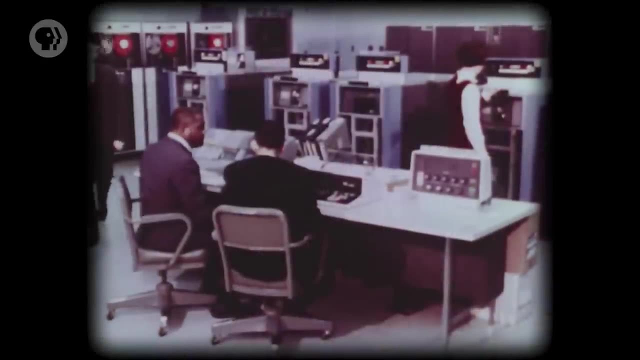 The continuous nature of tape made it easy to handle mechanically and the holes could be reliable and easy to use. But of course humans don't think in terms of little punch holes and strips of paper. So the burden was on the programmers. They had to spend the extra time and effort to 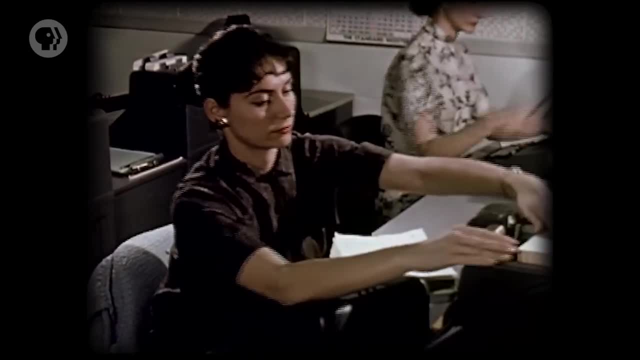 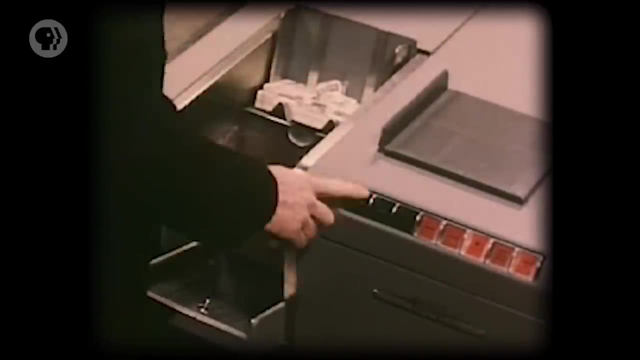 convert their ideas and programs into a language and a format that was easy for computers of the era to understand, often with the help of additional staff and auxiliary devices. It's also important to note that early computers- basically pre-1950, had an extremely simple 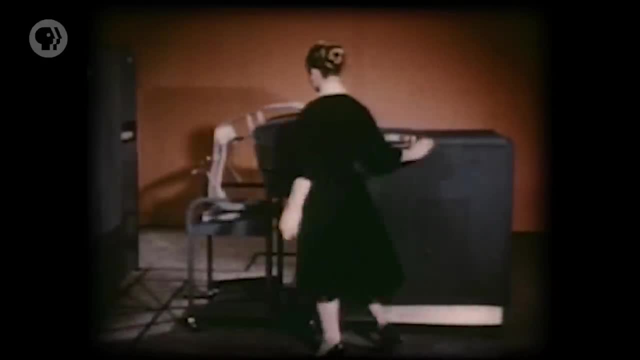 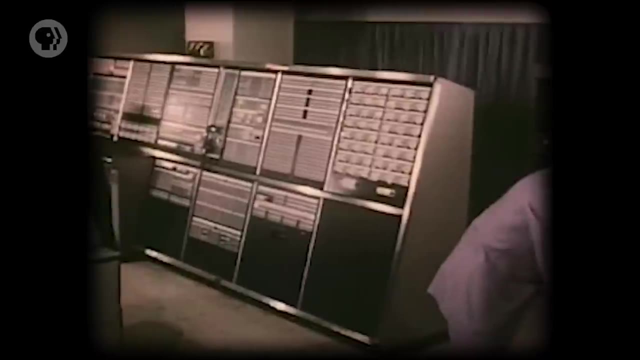 notion of human input. Yes, humans input programs and data into computers, But these machines generally didn't respond interactively to humans. Once a program was started, it typically ran until it was finished. That's because these machines were way too expensive to be waiting around for humans to type a command or enter. 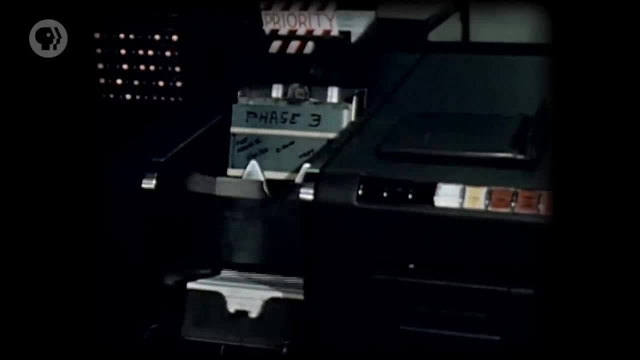 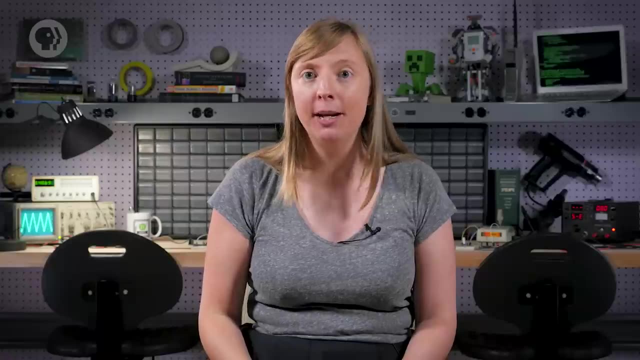 data. Any input needed for a computation was fed in at the same time as the program. This started to change in the late 1950s. On one hand, smaller-scale computers started to become cheap enough that it was feasible to have a human in the loop – that is a. 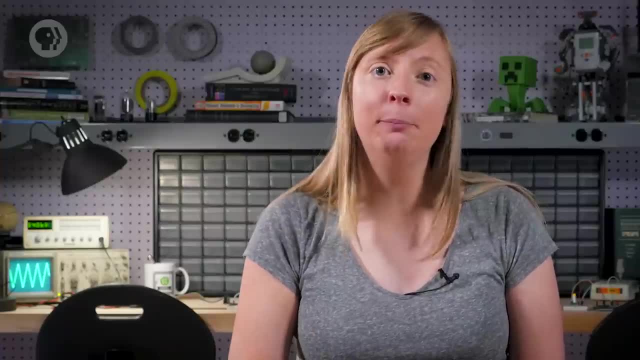 back-and-forth between human and computer And, on the other hand, smaller-scale computers started to become cheap enough that it was feasible to have a human in the loop. That is a back-and-forth between human and computer. On the other hand, big, fancy computers became fast and sophisticated enough to support many. 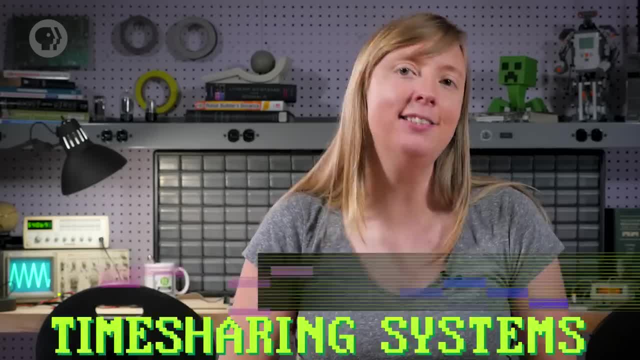 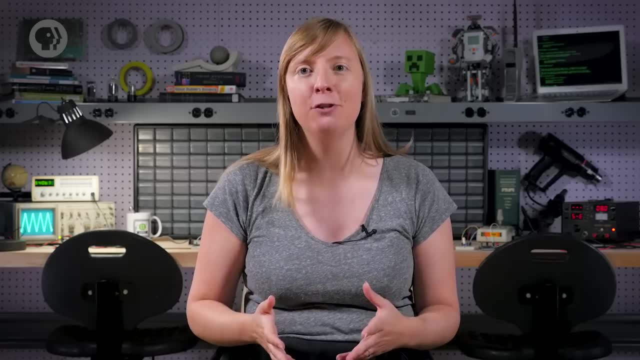 programs and users at once – what were called multitasking and timesharing systems. But these computers needed a way to get input from users. For this, computers borrowed the ubiquitous data entry mechanism of the era – keyboards At this point. typing machines had already been in use for a few centuries, But it was 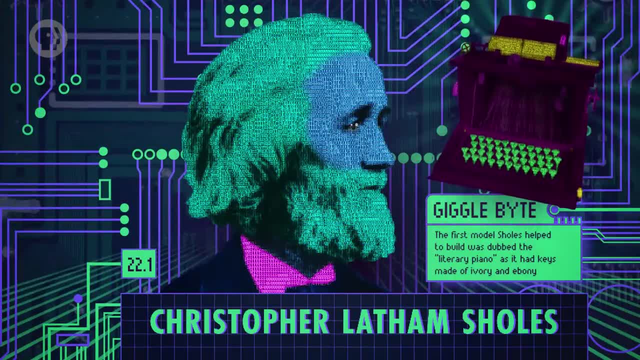 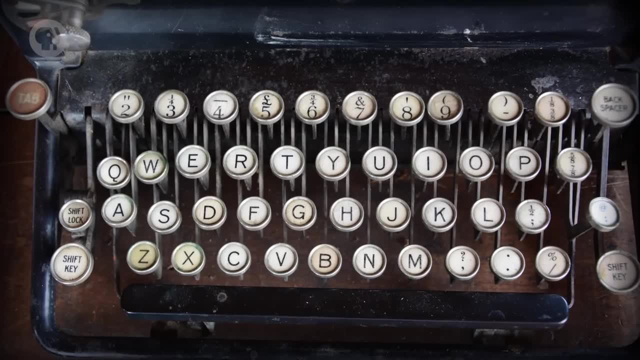 Christopher Latham Sholes, who invented the modern typewriter in 1868.. It took until 1874 to refine the design and manufacture it, but it went on to be a commercial success. Sholes' typewriter adopted an unusual keyboard layout that you know well – QWERTY named. 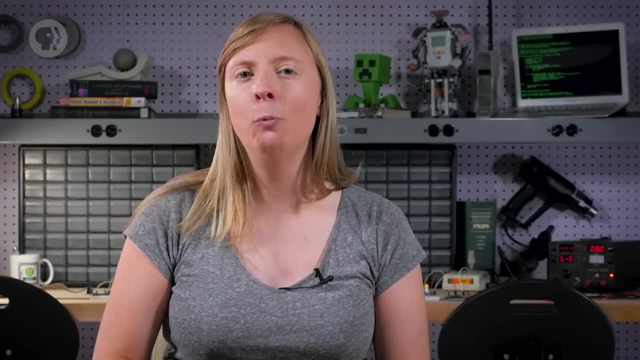 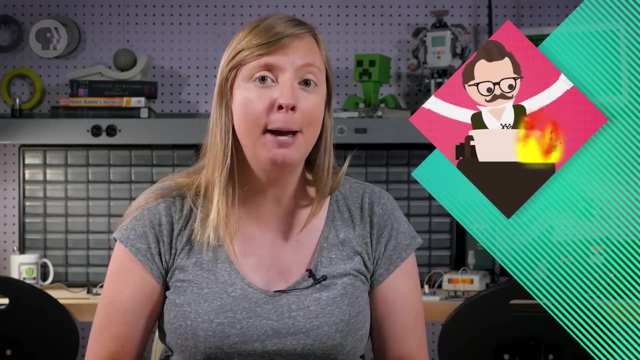 for the top-left row of letter keys. There has been a lot of speculation as to why this design was used. The most prevalent theory is that it put common letter pairings in English far apart to reduce the likelihood of type bars jamming when entered in sequence. 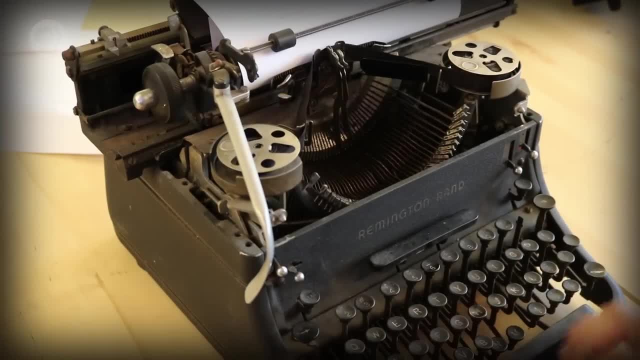 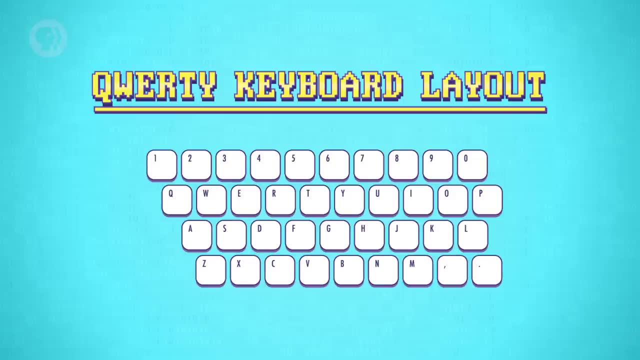 It's a convenient explanation, but it's also probably false – or at least not the full story. In fact, QWERTY puts many common letter pairs together, like TH and ER, And we know that Sholes and his team went through a lot of trouble to come up with a way to. 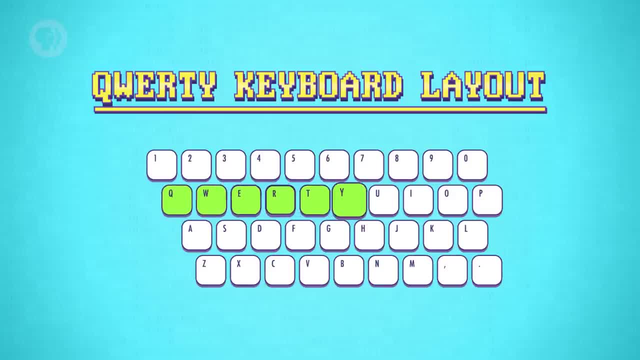 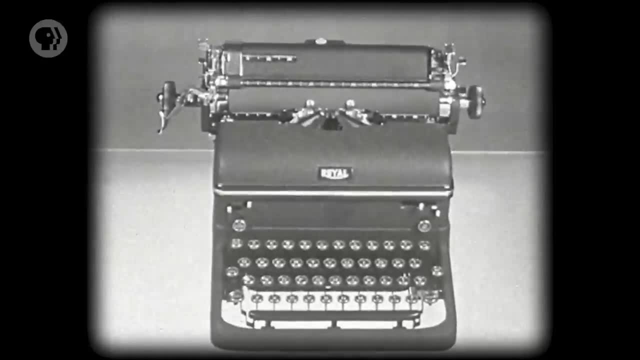 make this iconic keyboard layout, In fact, the first time. Sholes and his team went through many iterations before arriving at this iconic arrangement. Regardless of the reason, the commercial success of Sholes' typewriter meant that the competitor companies that soon followed duplicated his design. Many alternative keyboard layouts. 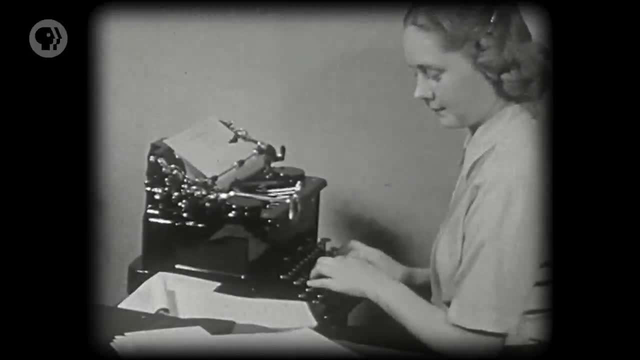 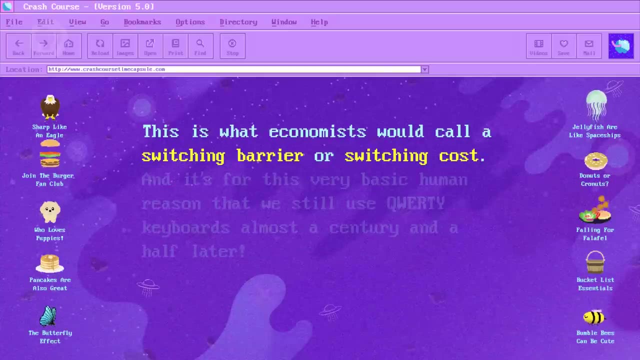 have been proposed over the last century, claiming various benefits, But once people had invested the time to learn QWERTY, they just didn't want to learn something new. This is what economists would call a switching barrier or switching cost, And it's for. 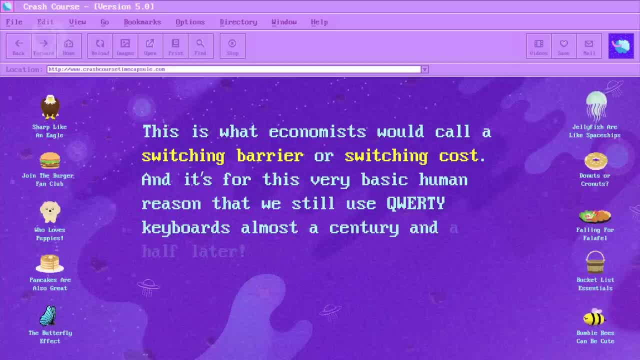 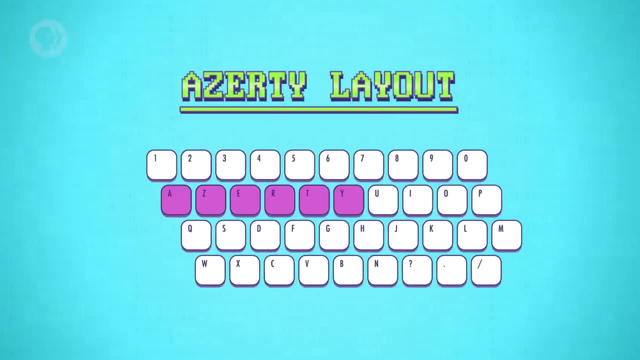 this very basic human reason that we still use QWERTY keyboards almost a century and a half later. Not to mention that QWERTY isn't universal. There are many international variants, like the French AZERTY layout or the QWERTZ layout common in Central Europe. 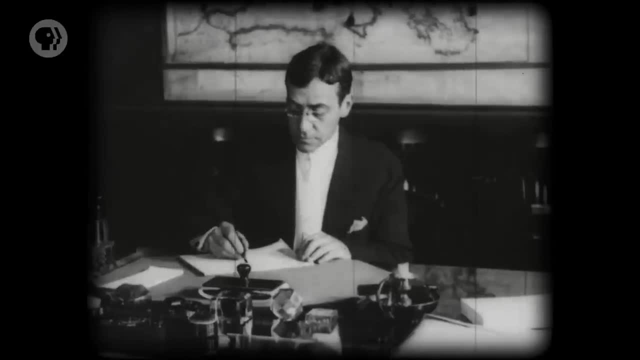 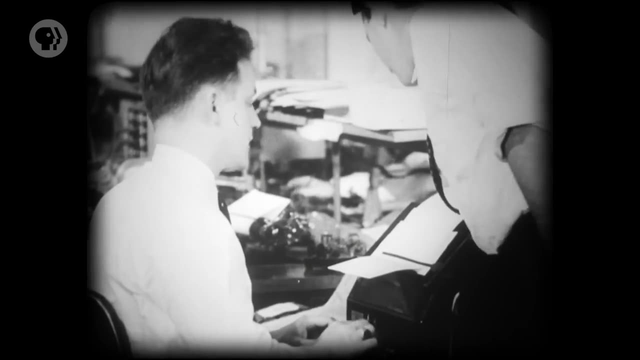 Interestingly, Sholes didn't envision that typing would ever be faster than handwriting, which is around 20 words per minute. Typewriters were introduced chiefly for legibility and standardization of documents, not speed. However, as they became standard equipment in offices. 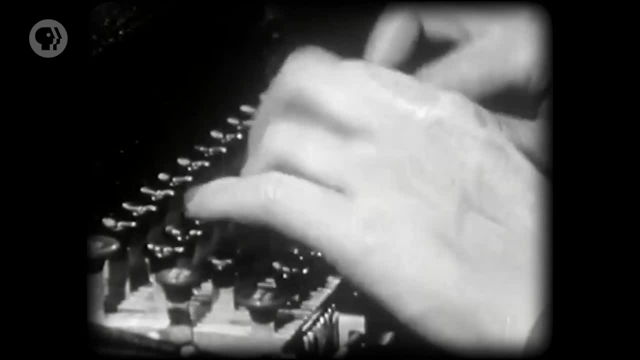 the desire for speedy typing grew, And there were two big advances that unlocked typing's true potential. Elizabeth Longley, a teacher at the Cincinnati School of Mathematics, was a teacher at the University of Cincinnati in 1880.. Around 1880,, Elizabeth Longley, a teacher at the Cincinnati 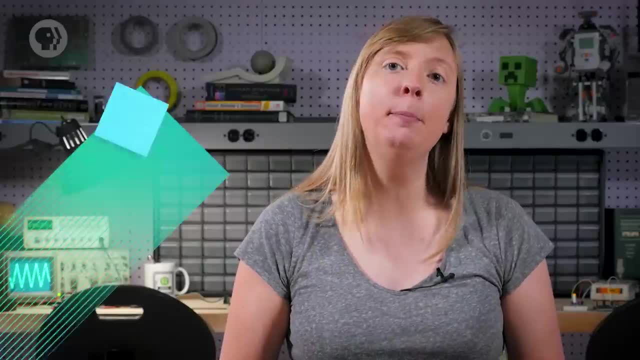 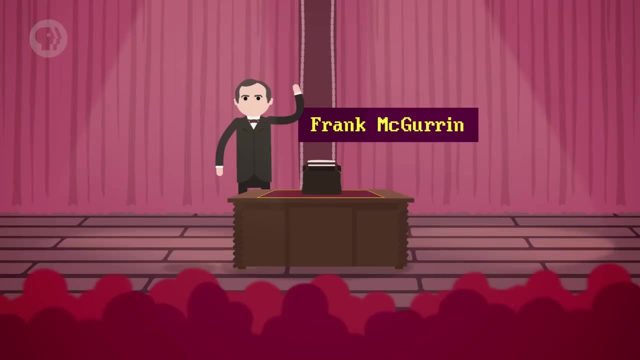 Shorthand and Typewriter Institute started to promote ten-finger typing. This required much less finger movement than the Hunt and Peck, so it offered enhanced typing speeds. Then, a few years later, Frank McGurin, a federal court clerk in Salt Lake City, taught himself. 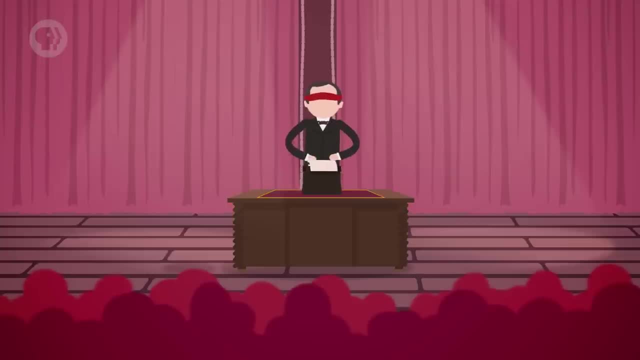 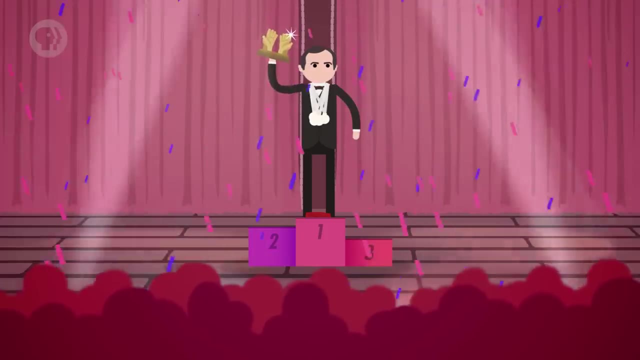 to touch type. As in, he didn't need to look at the keys while typing. In 1888, McGurin won a highly publicized typing speed contest, after which ten-finger touch typing began to catch on. Professional typists were soon able to achieve speeds upwards of 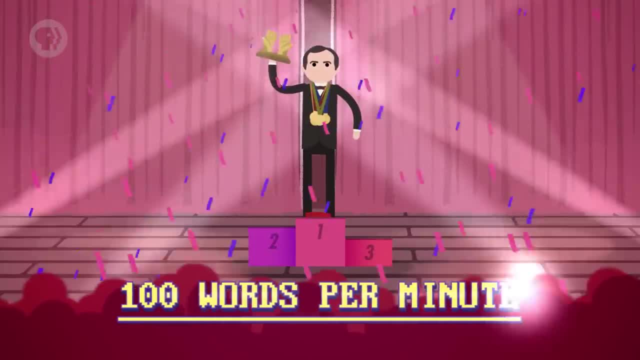 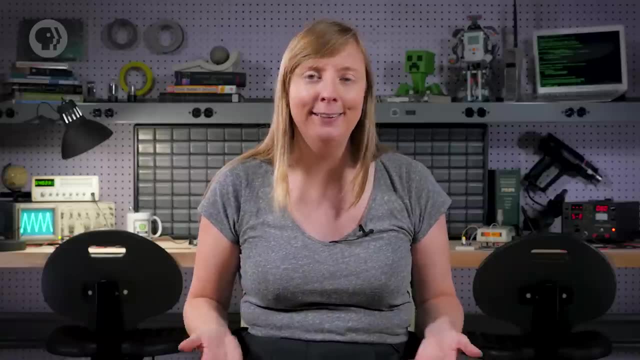 a hundred words per minute, Much faster than handwriting, and nice and neat too. So humans are pretty good with typewriters. But we can't just plunk down a typewriter in front of a computer and have it type. They have no fingers. 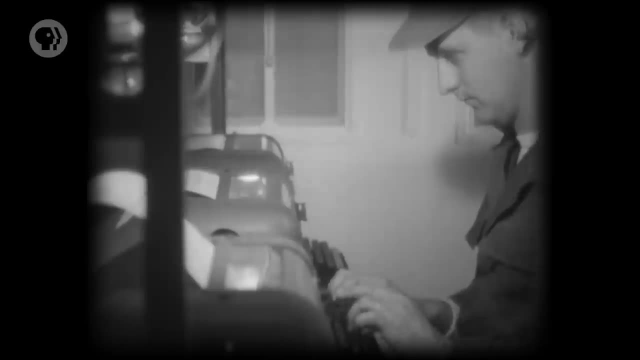 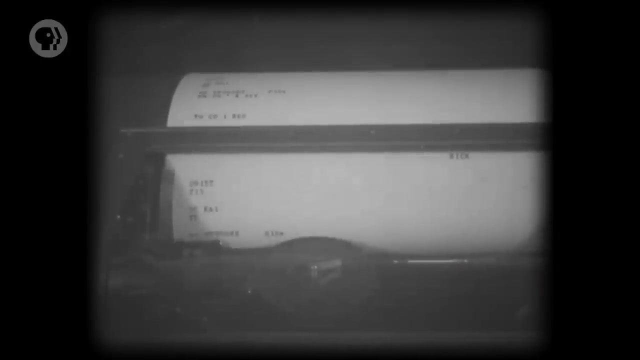 Instead, early computers adapted a special type of typewriter that was used for telegraphs, called a teletype machine. These were electromechanically augmented typewriters that could send and receive text over telegraph lines. Pressing a letter on one teletype keyboard would cause 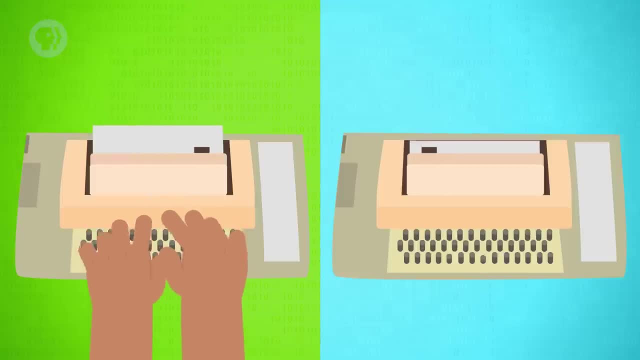 a signal to be sent over telegraph wires to a teletype machine on the other end, Which would then electromechanically type that letter. This allowed two humans to type to one another over long distances- Basically a steampunk version of a chat room. 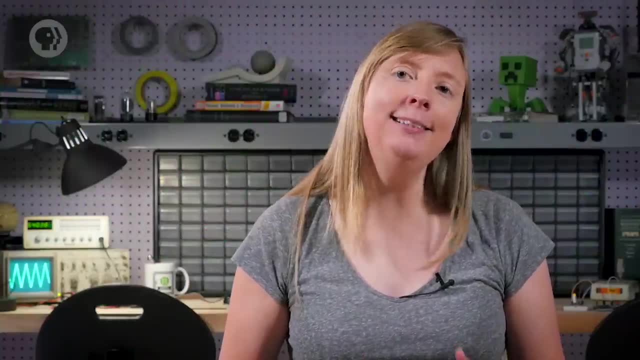 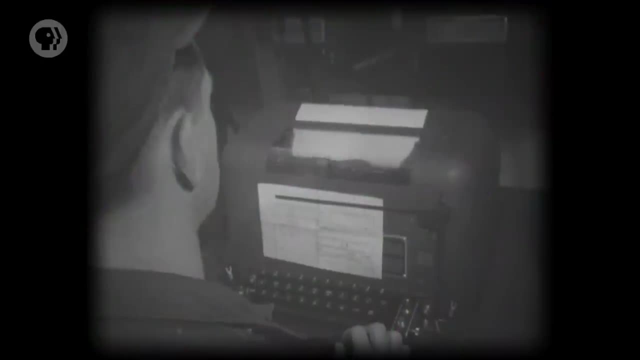 Since these teletype machines already had an electronic interface, they were easily adapted for computer use, And teletype computer interfaces were common in the 1960s and 70s. Interaction was pretty straightforward: Users would type a command, hit enter and then. 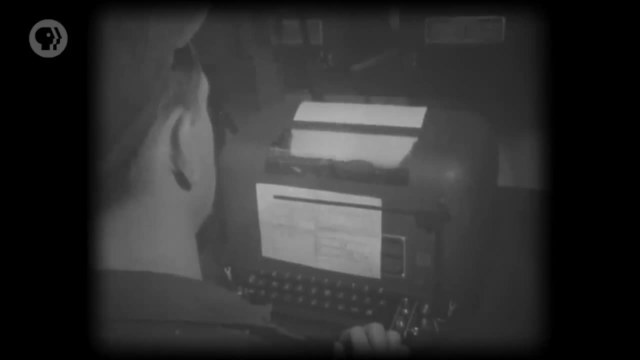 the computer would type back This text. CONVERSATION between a user and a computer went back and forth. These were called telegraphs, These were called telegraphs, These were called telegraphs, These were called command line interfaces, and they remained the most prevalent form. 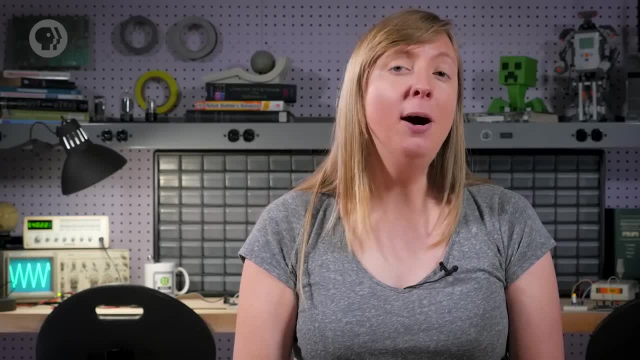 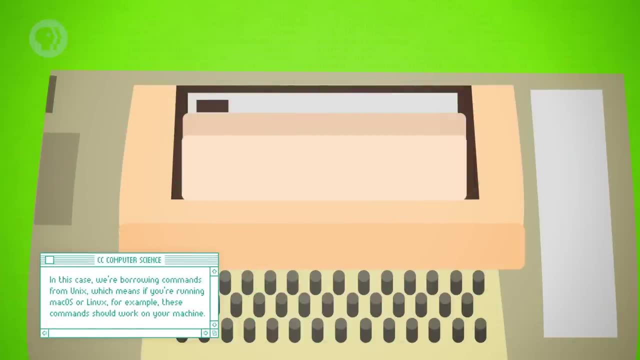 of human-computer interaction up until around the 1980s. Command line interaction on a teletype machine looks something like this: A user can type any number of possible commands. Let's check out a few, beginning with seeing all the files in the current directory we're in. 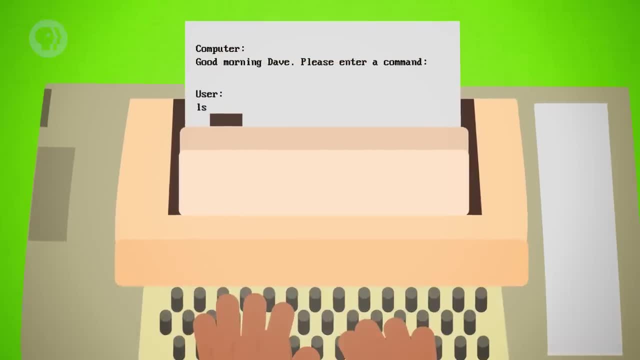 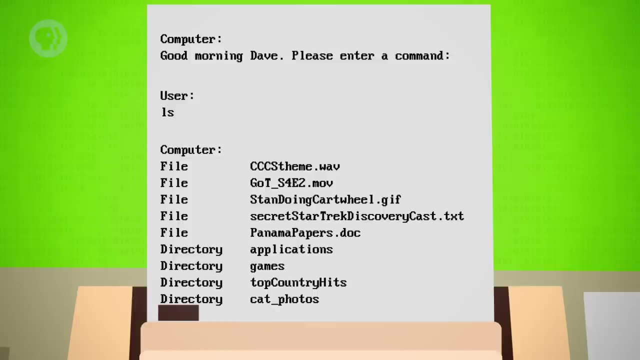 For this we would type the command ls, which is short for list, and the computer replies with a list of the files in our current directory. If we want to see what's in our secret Star Trek Discovery Cast dot txt file we use. yet 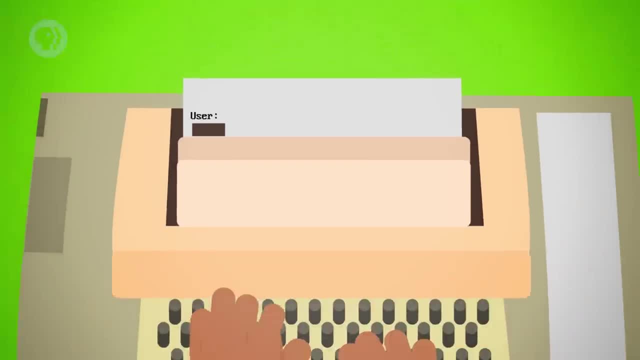 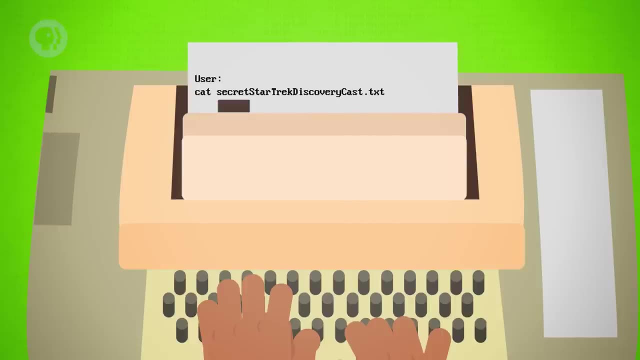 another command to display the contents. In Unix we can call cat, short for concatenate. We need to specify which file to display, so we include that after the command called an argument. If you're connected to a network with other users, you can use a primitive version of. 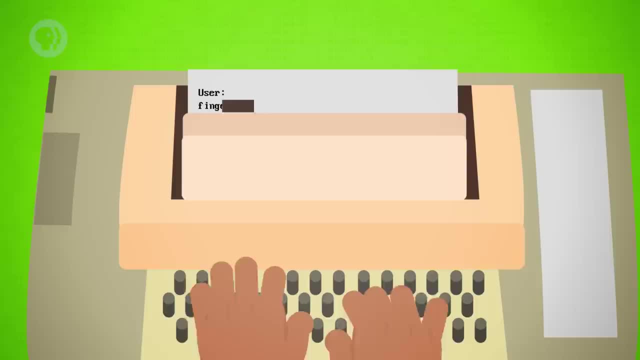 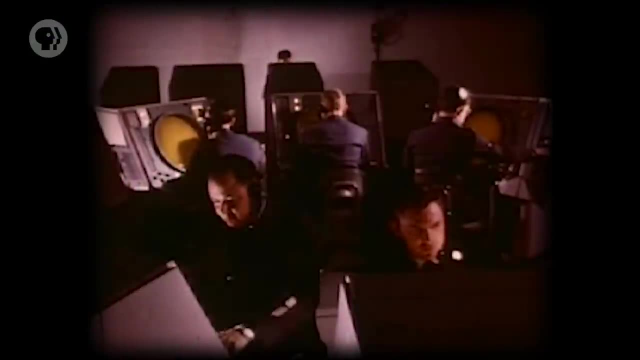 a Find My Friends app to get more info on them. with the command finger, Electro-mechanical teletype machines were the primary computing interface for most users up until around the 1970s, Although computer screens first emerged in the 1950s and were 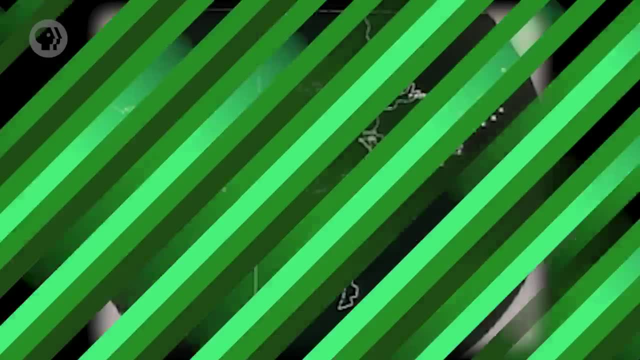 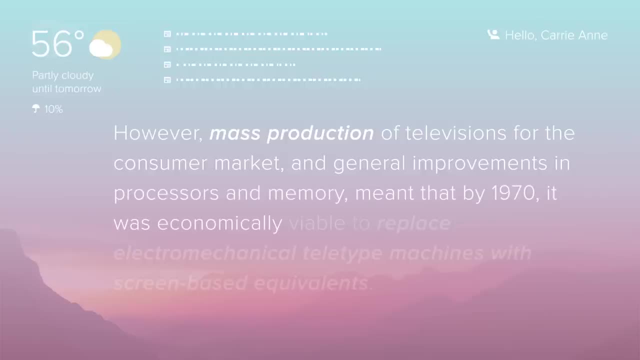 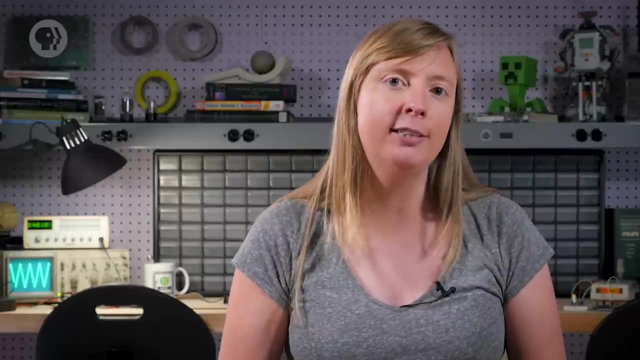 used for graphics they were too expensive and low resolution for everyday use. However, televisions for the consumer market and general improvements in processors and memory meant that by 1970 it was economically viable to replace electro-mechanical teletype machines with screen-based equivalents, But rather than build a whole new standard to interface. 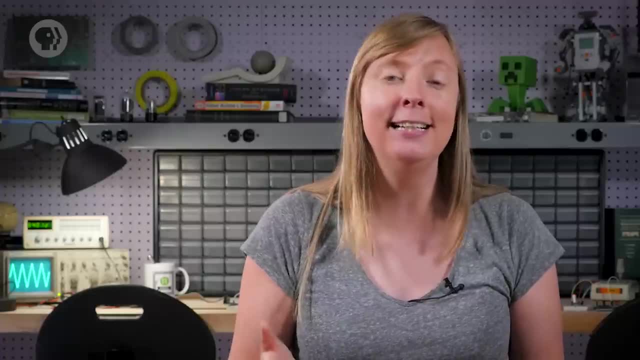 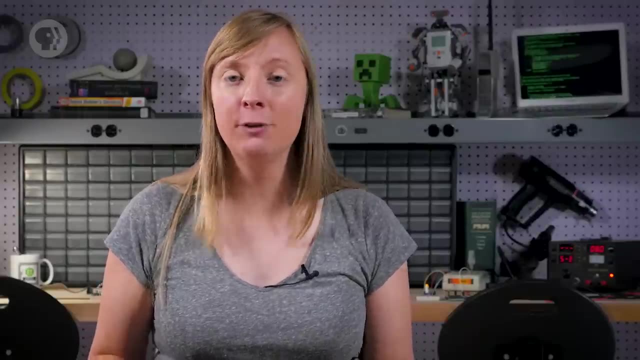 computers with these screens. engineers simply recycled the existing text-only teletype protocol. These machines used a screen which simulated endless paper. It was text in and text out, nothing more. The protocol was identical, so computers couldn't even tell if it was. 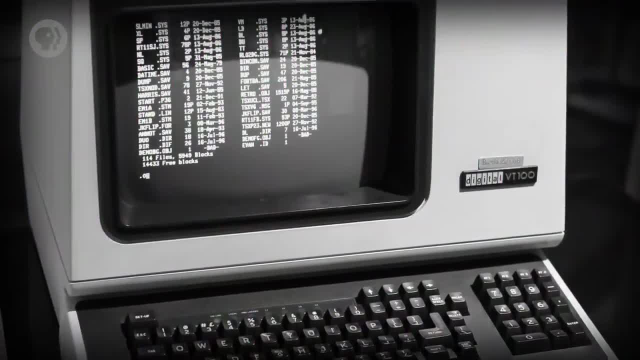 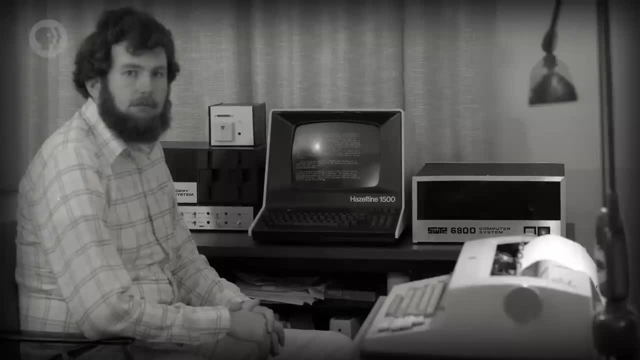 paper or a screen. These virtual teletype or glass teletype machines became known as terminals. By 1971, it was estimated in the United States there was something on the order of 70,000 electro-mechanical teletype machines and 70,000 screen-based terminals in use. 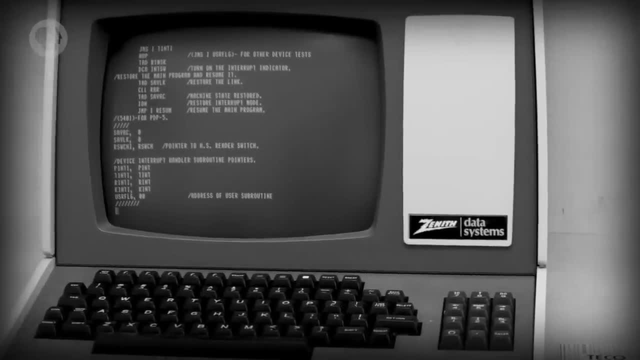 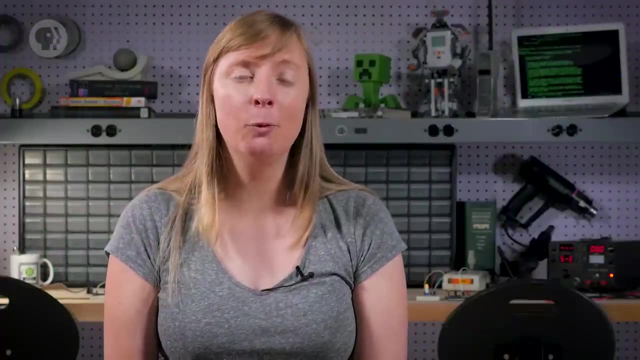 Screens were so much better, faster and more flexible, though, Like you, could delete a mistake and it would disappear. So by the end of the 1970s, screens were standard. You might think that command-line interfaces are way too primitive to do anything interesting. 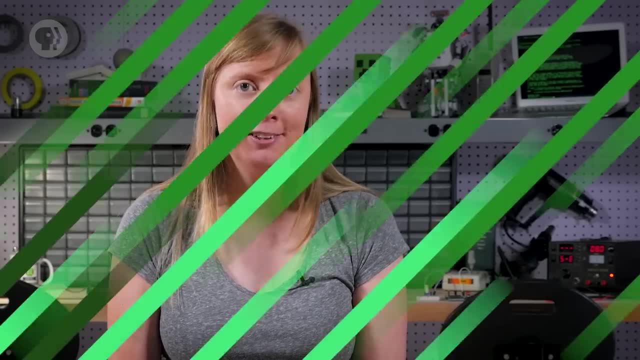 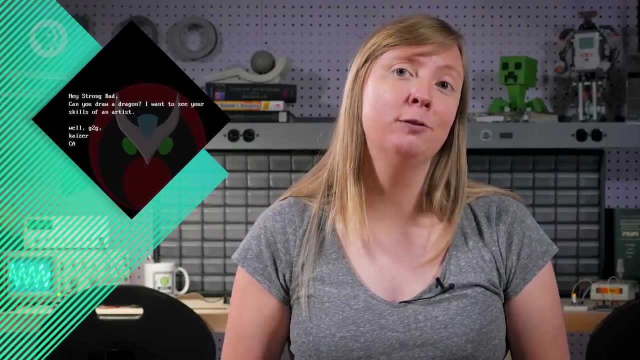 But even when the only interaction was through text, programmers found a way to make them fun. Early interactive text-based computer games include famous titles like Zork, created in 1977. Players of these sorts of early games were expected to engage their limitless imaginations. 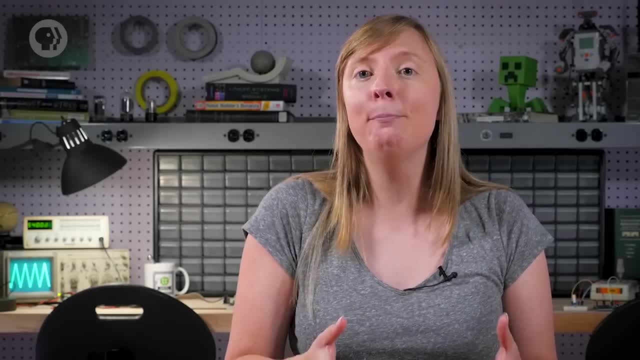 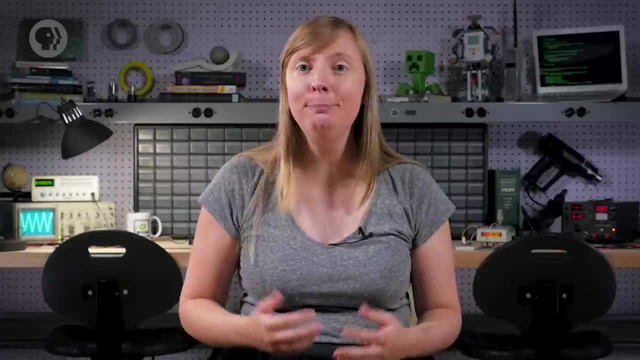 as they visualized the fictional world around them, Like what terrifying monster confronted them when it was pitch black and you were likely to be eaten by a grue. Let's go back to our command line now on a fancy screen-based terminal, and play. 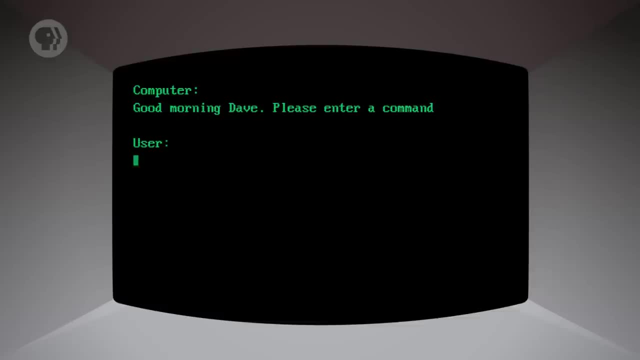 Just like before, we can see what's in our current directory with the ls command. Then let's go into our games directory by using the cd command. Let's go back to our games directory by using the cd command. Let's go back to our games directory by using the cd command. 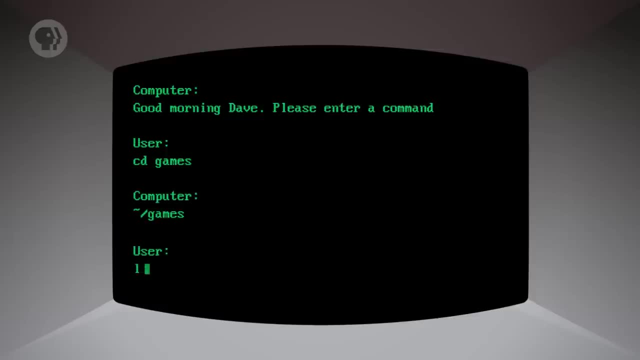 Let's go back to our games directory by using the cd command. Now we can use our ls command again to see what games are installed on our computer. Sweet, We have adventure. All we have to do to run this program is type its name. Until this application halts or 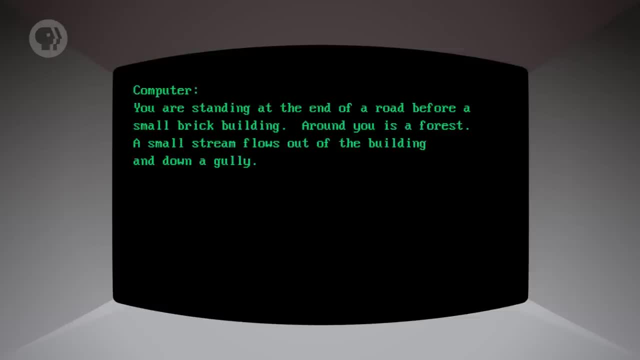 we quit it, it takes over the command line. What you're seeing here is actual interaction from Colossal Cave Adventure, first developed by Will Crowther in 1976.. In the game, players can type in one- or two-word commands to move. 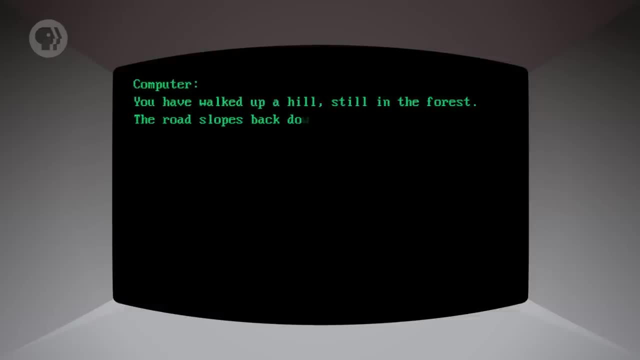 around, interact with objects, pick up items and so on. The program acts as the narrator, describing locations, possible actions and mechanisms. actions and the results of those actions. Certain ones resulted in death. The original version only had 66 locations to explore, but it's widely considered to. 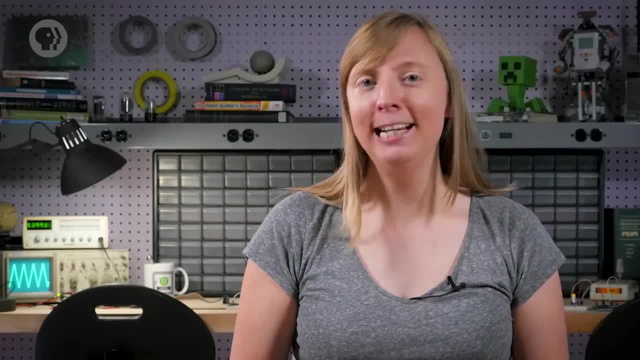 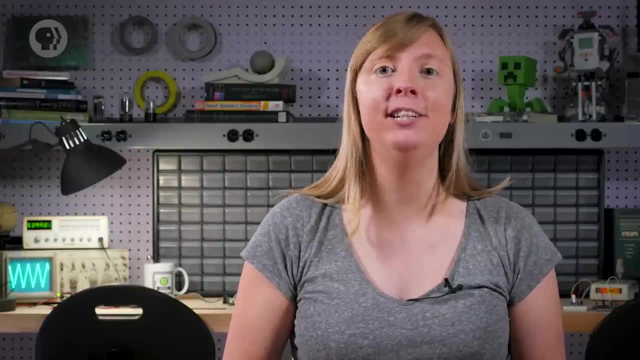 be the first example of interactive fiction. These text adventure games later became multiplayer, called MUDs or multi-user dungeons, And they're the great forbearers of the awesome graphical MMORPGs we enjoy today. And if you want to know more about the history of these and other games, we've got a whole 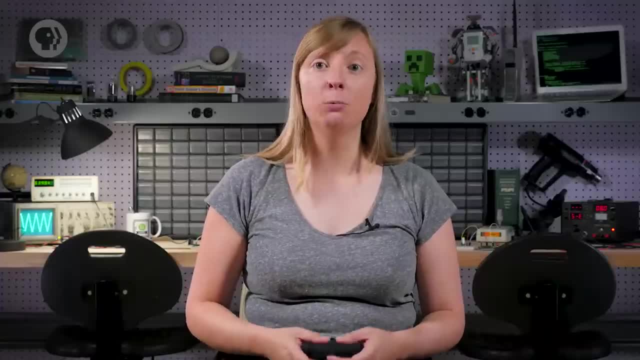 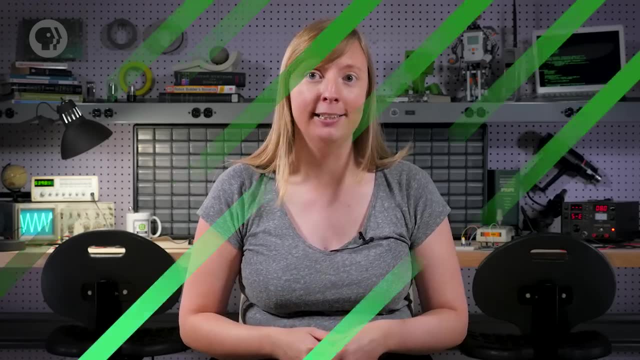 series on it hosted by Andre Meadows. Command line interfaces, while simple, are very powerful. Computer programming is still very much a written task and, as such, command lines are a natural interface. For this reason, even today, most programmers use command line interfaces as part of their 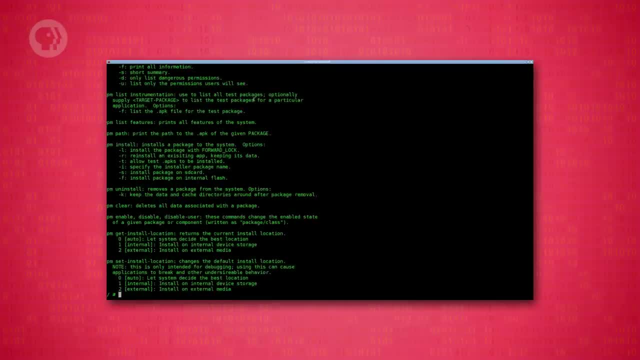 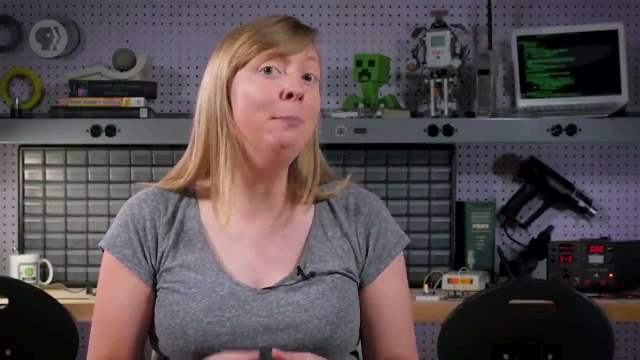 work, And they're also the most common way to access computers that are far away, like a server in a different country. If you're running Windows, MacOS or Linux, your computer has a command line interface, one you may have never used. 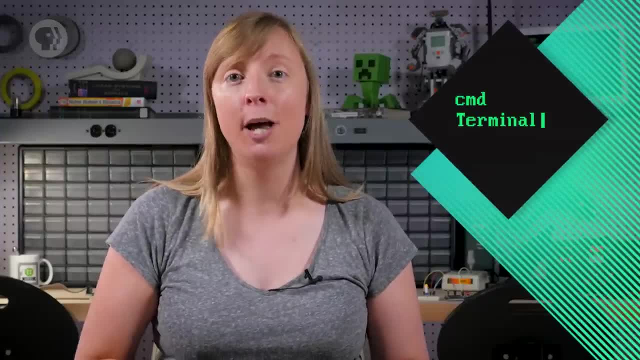 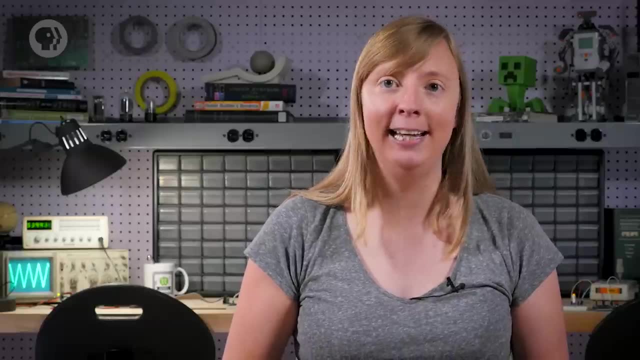 Check it out by typing CMD in your Windows search bar or search for Terminal on Mac. Then install a copy of Zork and play on. So you can see how these early advancements work. And if you want to know more about the history of digital studios, check out our video on. 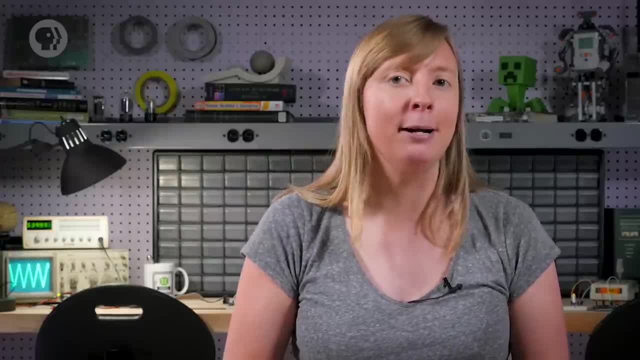 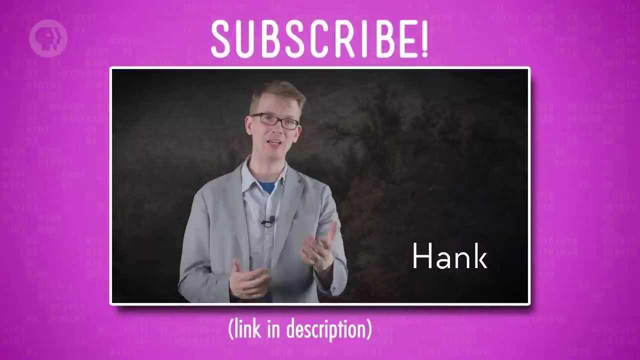 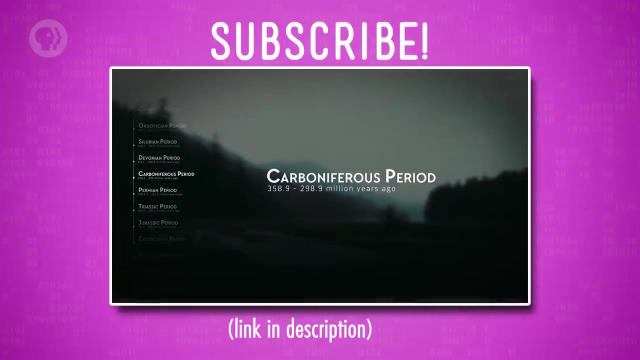 the Internet. But before we go, I wanted to tell you about a new show produced by Complexly and PBS Digital Studios: Eons. Eons is about exploring the history of life on Earth all the way up to the most recent ice age and, yes, dinosaurs.